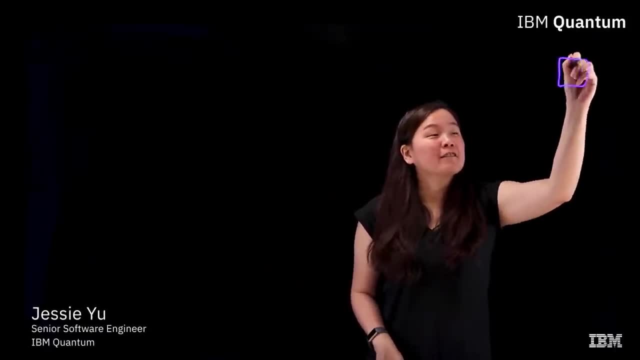 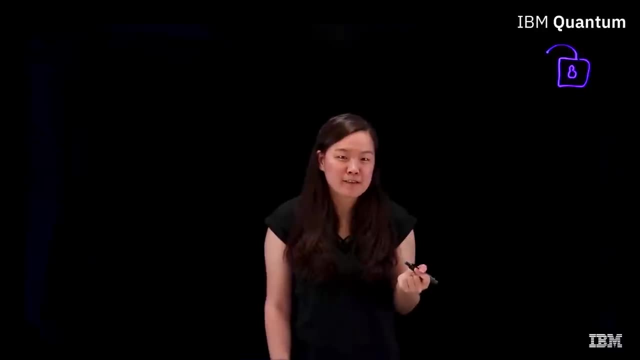 An ideal quantum computer can break the encryption standards we use today by finding prime factors of a large integer in just minutes instead of the thousands of years it would take for a classical computer to do. But before you start to panic, while we have real quantum, 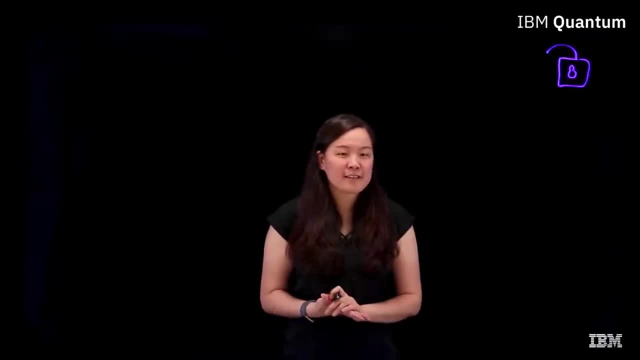 hardware today, it's not quite powerful enough to do that just yet. However, technologies are advancing faster than ever. The cell phones we have today are more powerful than the membranes that we use to send people to the moon, And the researchers believe that we will soon. 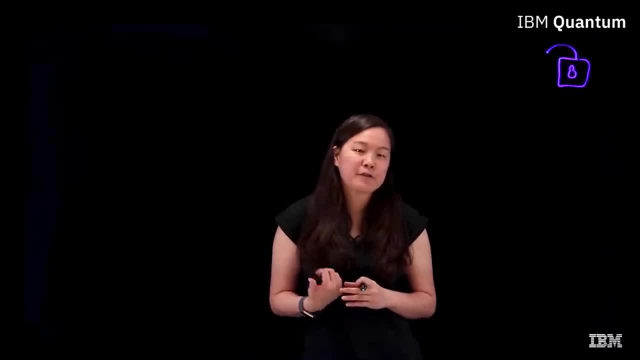 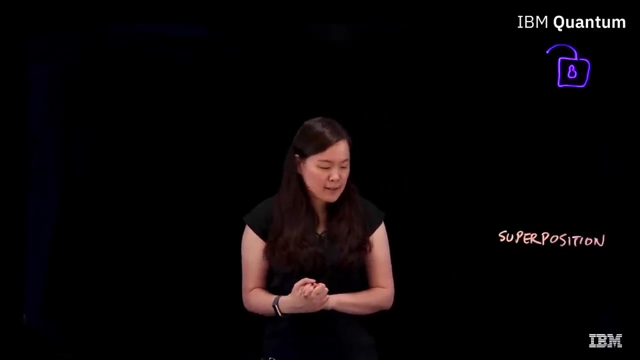 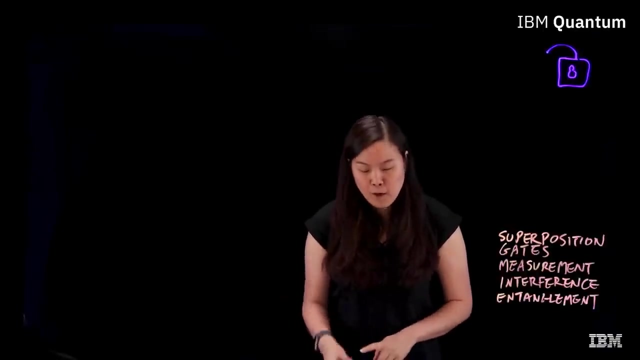 enter an era of quantum advantage, where quantum computers will be used to accelerate classical computers, just like GPUs. In this video I'm going to talk about five foundational topics in quantum computer: Superposition: gates, measurement, interference and entanglement. 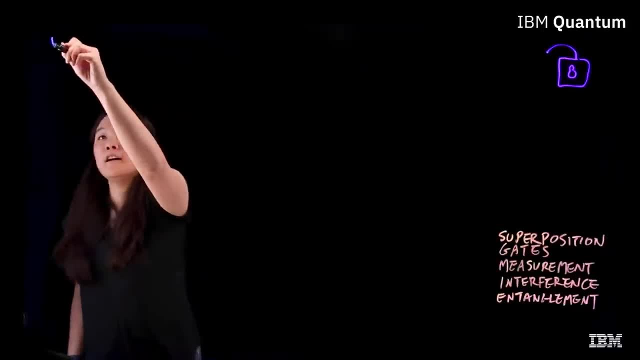 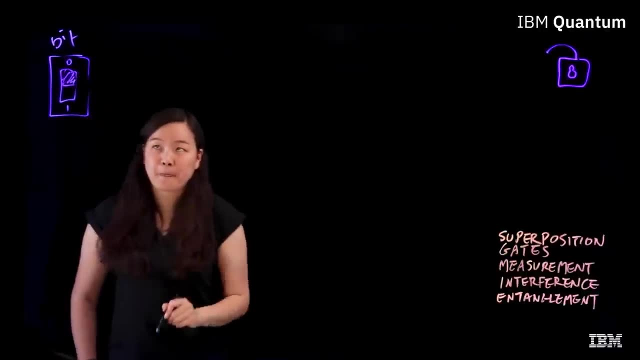 But before we dive into that, let's first talk about bits. Classical computers use bits, which are like switches That can be a 0 or a 1.. This way of computation has served us well, So well, in fact, that almost all modern computers. 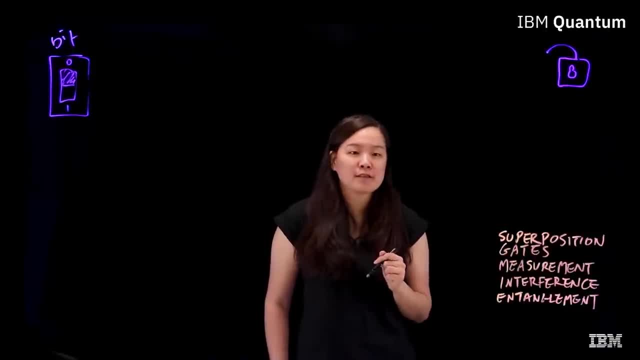 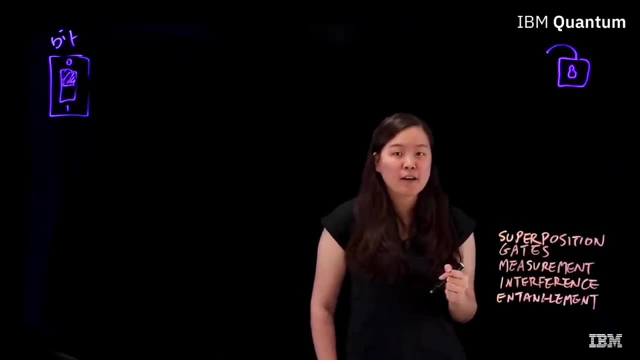 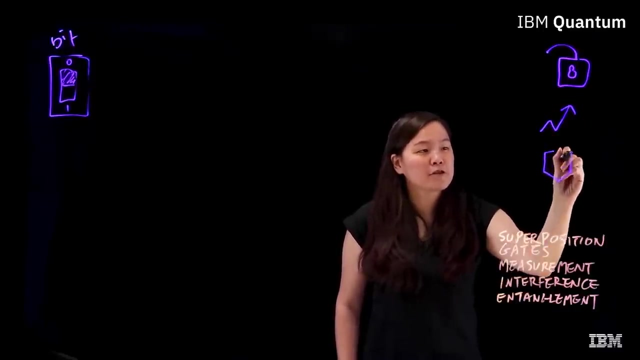 work this way. However, this approach doesn't solve all the problems that we have, Problems that can blow up exponentially and would take classical computers decades or more to solve. We already talked about the algorithm we use for encryption. Other types of difficult problems include optimization, chemistry, simulation and machine learning. 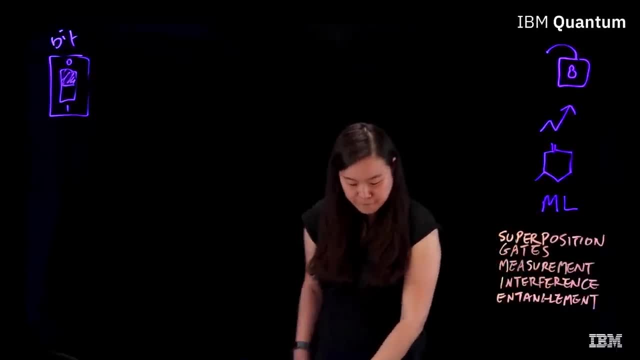 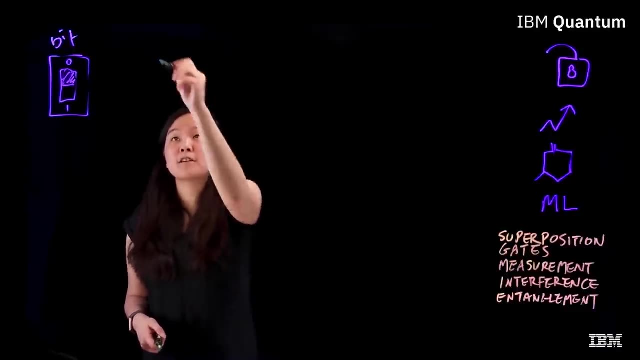 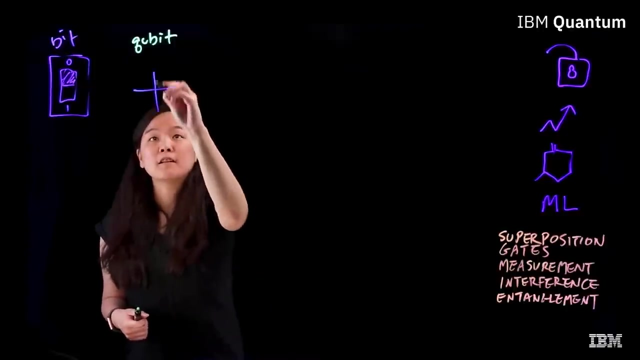 Now let's talk about our first topic: superposition. Quantum computer does not use this simple 0 and 1 bits. Instead it uses qubits. A qubit can be a 0,, a 1, or any linear combination of the two. This spectrum of states is what 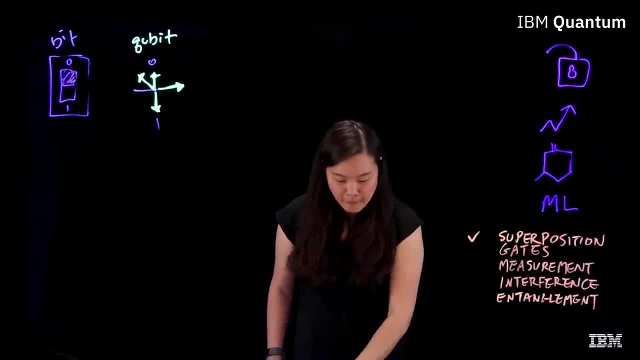 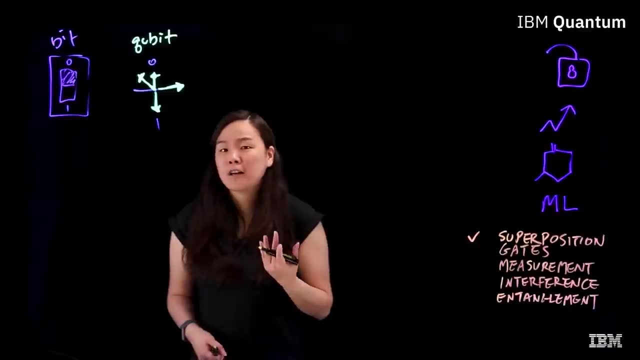 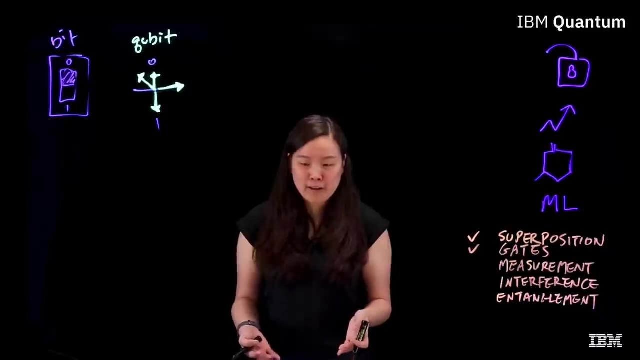 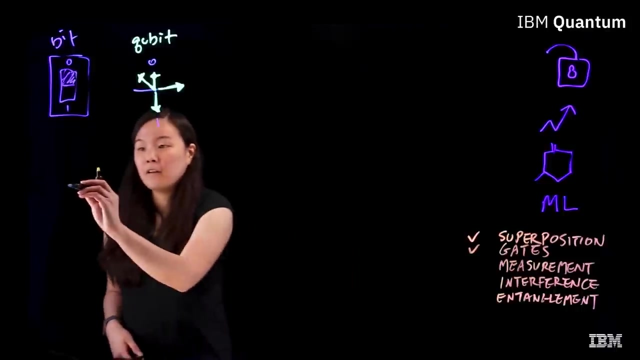 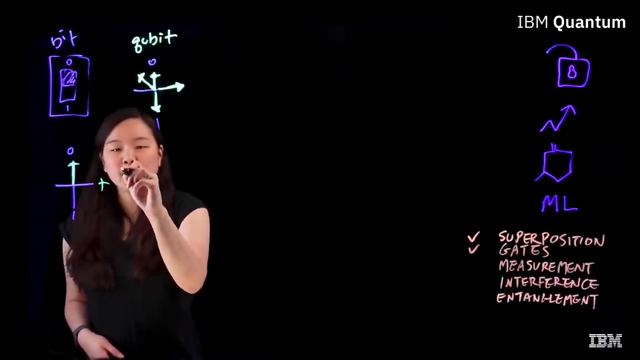 we call a superposition. Our next topic topic is about gates. Similar to classical computers, we string together qubits using a construct called gates that can alter the state of qubits in a circuit. For example, we can have a qubit that's at the state of zero, Then we can use the Hadamard gate or 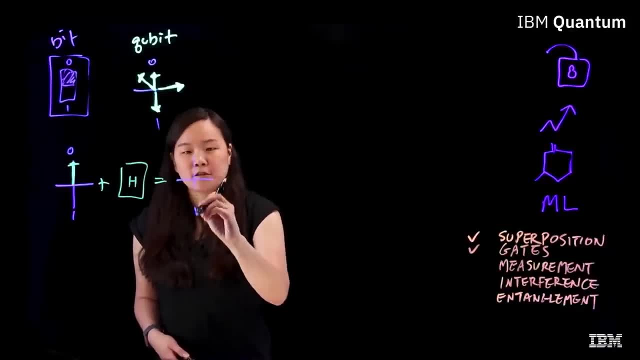 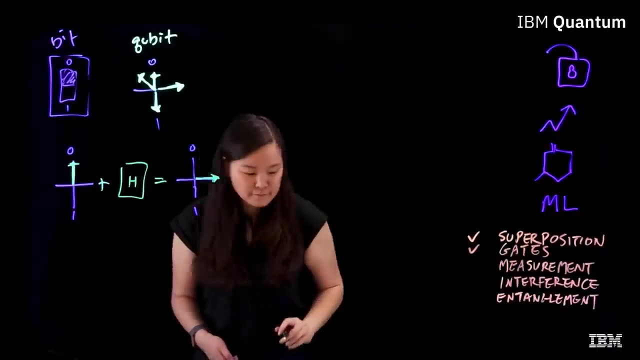 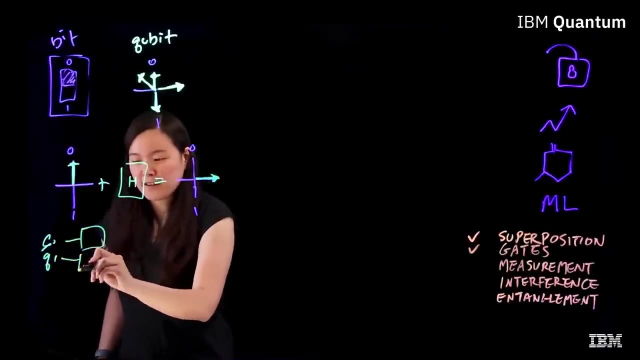 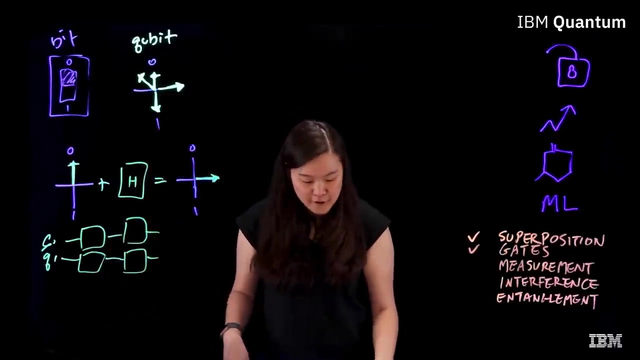 H-gate for short, to put it in a superposition between zero and one. And of course, you can have multiple qubits with multiple gates in a circuit. For the circuit to be useful at some point you need to read about its outputs, which. 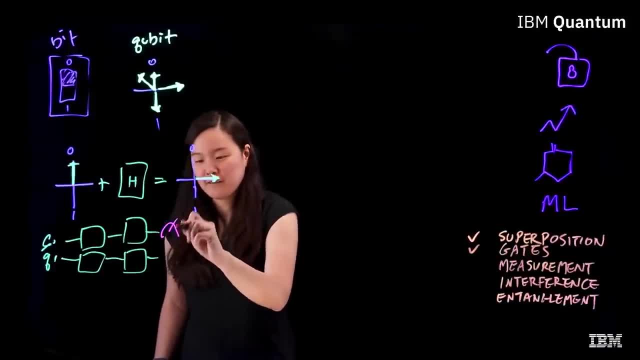 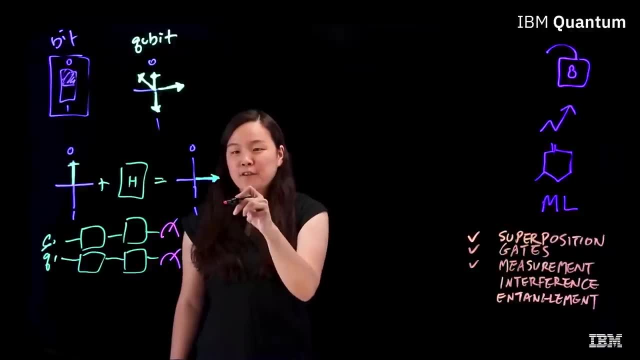 brings us to the next slide. Let's move on to our next topic: measurement. When a qubit is measured, it loses its superposition and collapses into just a simple 0 or 1.. That means an arrow pointing this way does not measure a 0.5.. Instead, it has a 50% chance. 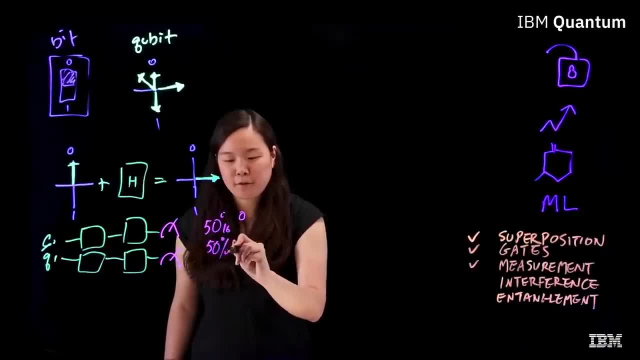 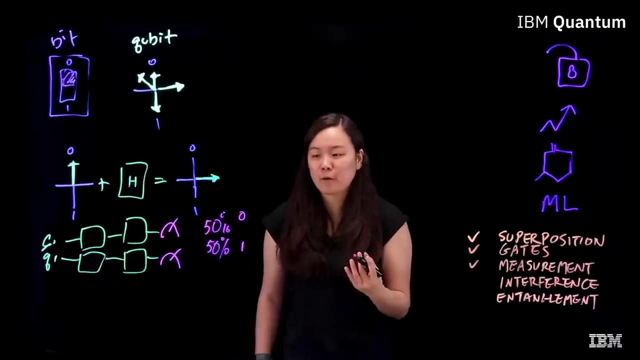 of measuring a 0 and 50% chance of measuring a 1.. It is this in-between state that allows a qubit to be a 0 and a 1 at the same time. It also means that just a small number of qubits can represent a large amount of information. 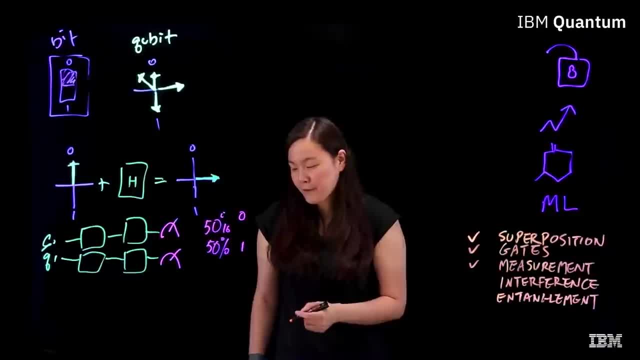 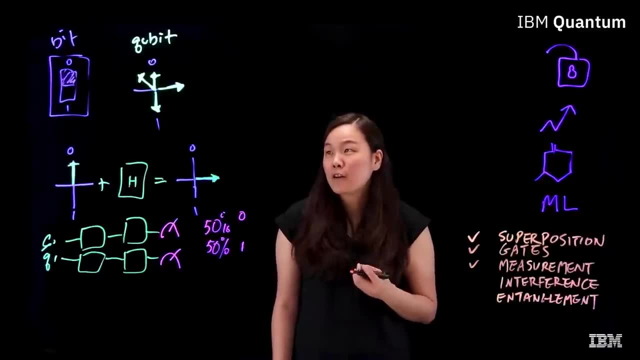 So for our next topic, interference, we begin by addressing a common question. Why is it that quantum computers can outperform classical ones? So if you read this slide, you can see that quantum computers can outperform classical ones. So if you read this slide, you can see that quantum computers can outperform classical ones. 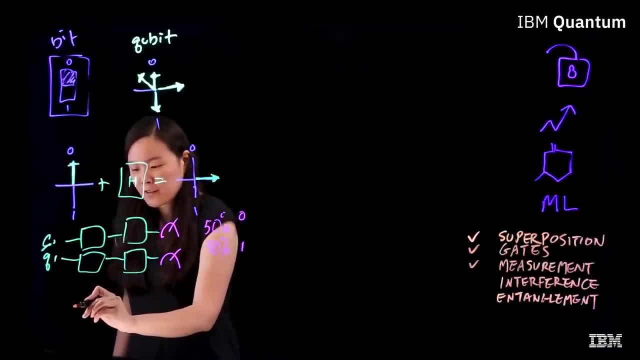 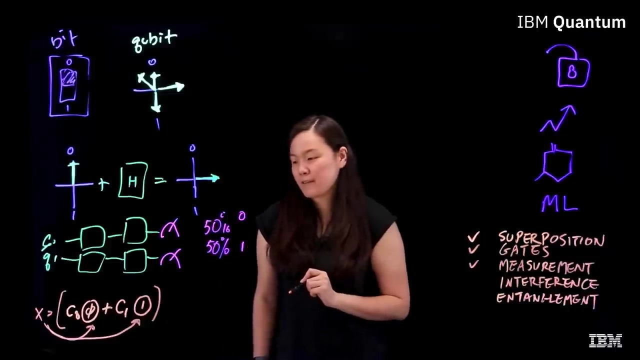 So, if you remember, a quantum state is a linear combination of the zero state and the one state. So an operation applied to this can be seen as applying to the zero state and the one state, doing two calculations at once. It is this parallel computation that gives quantum.